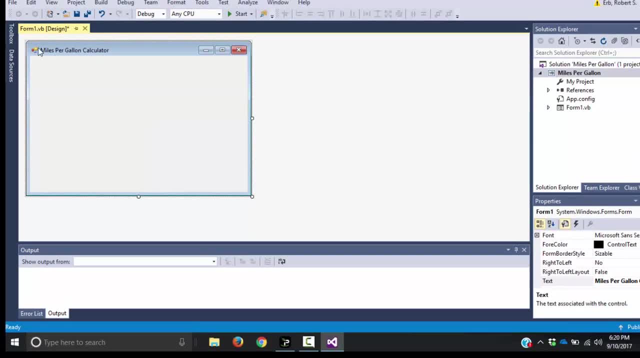 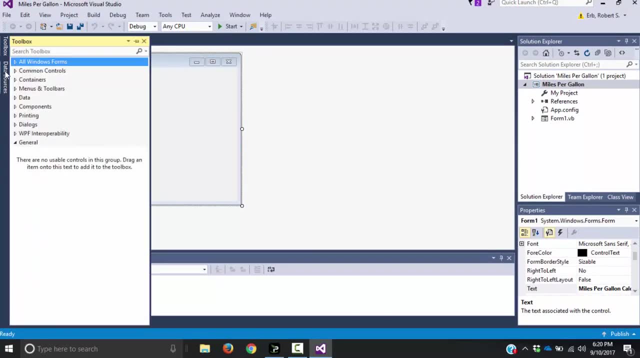 it'll look a little more professional. I need a button so the user can exit. That's always a good button to start with. So I'm going to click on my toolbox and you're going to get a little list that looks like this: I'm going to click on All Windows Forms just so I can see every. 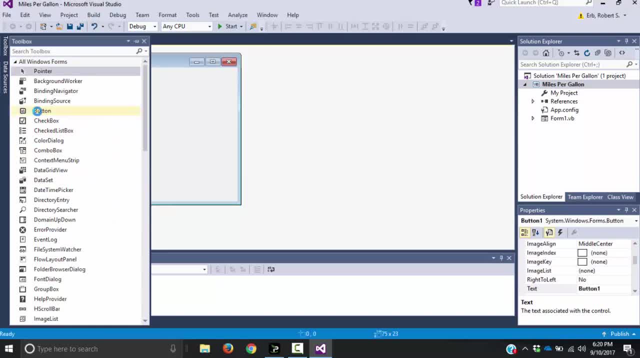 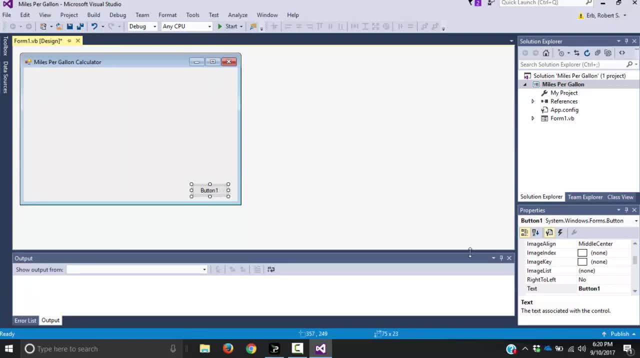 single tool that's available to me And I'm going to double click the button. I'm going to click back on my form. I see my button And the first thing I want to do is rename the name of this object. The text is what the button says, But I need to rename the. 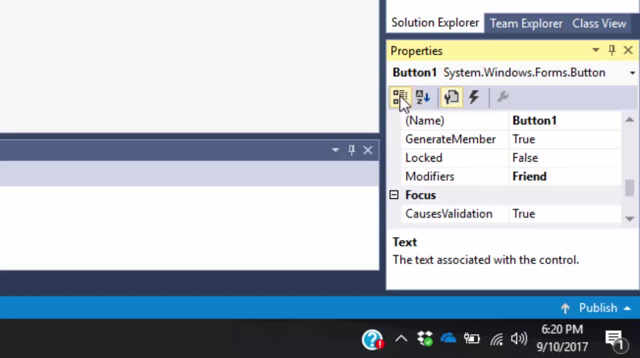 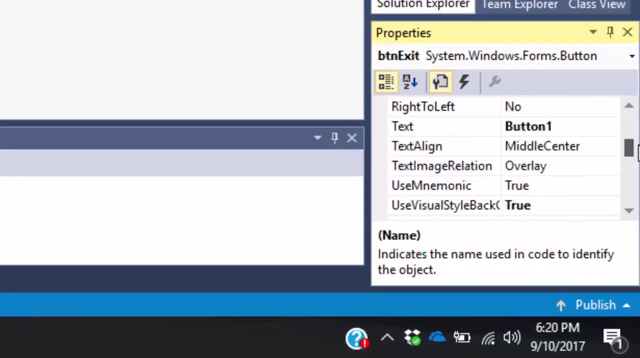 actual object, which is the button. So I scroll down to the name field in my properties window And the prefix we use for button is always btn And I'm going to call this exit. Now what I need to do is actually change the text of the button to say exit. That way the user 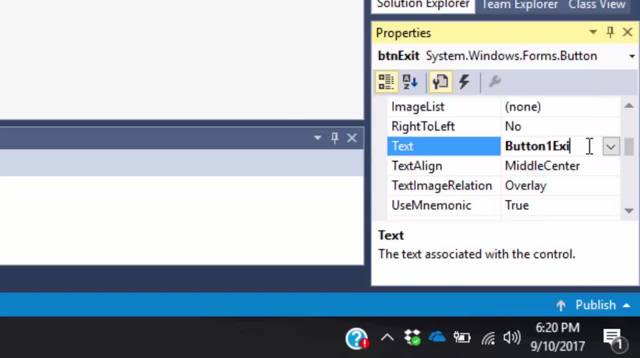 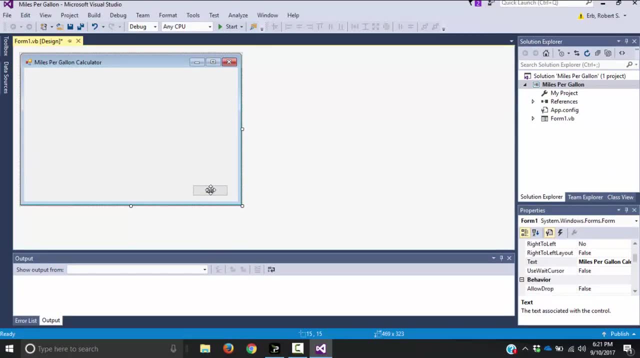 knows what it's actually doing. So I'm going to type in exit. All right, there we go. So this won't do anything. I've got to add some code. So what I'm going to do is I'm going to double click on the exit button, And what I'm going to do is I'm going to do application. 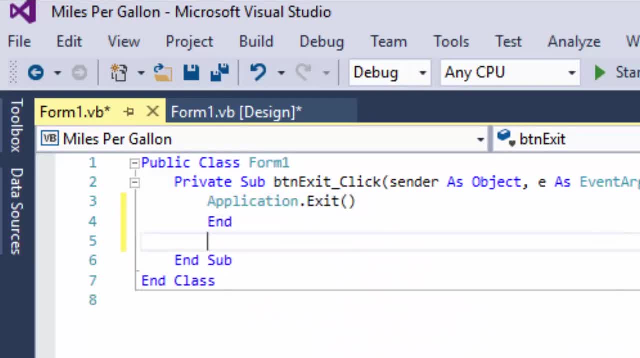 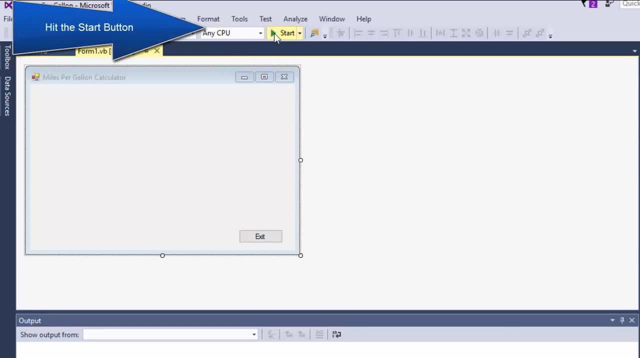 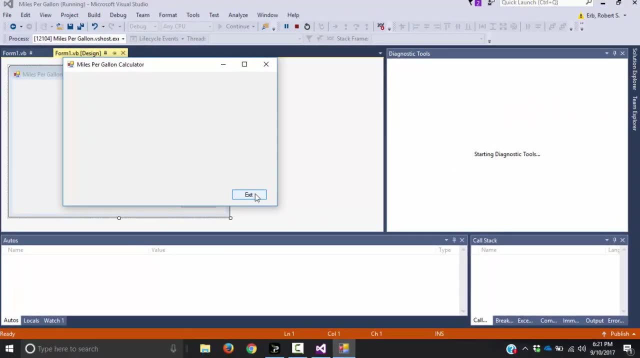 button, Dot, exit And then end, And what that will do is it will shut down my program So we can go ahead and do some testing real quick. It's going to build the program And we have the program here. I click on exit And it exits. So that's working. We said we were 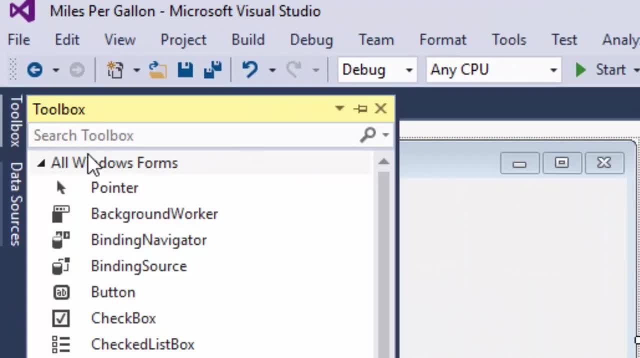 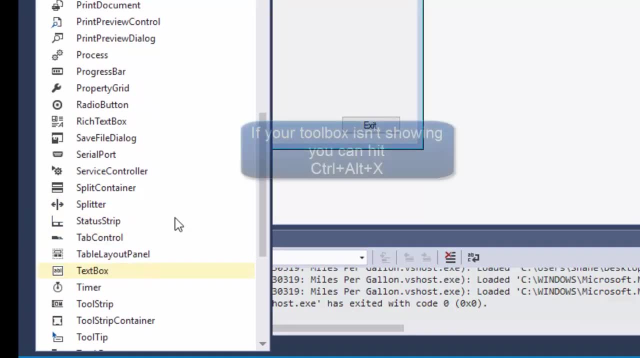 going to do a miles per gallon calculator, We need an input from the user. So I'm going to need a text box that they can actually input information into. So I'm going to need a text box, And what we can do is we can make this about the size. 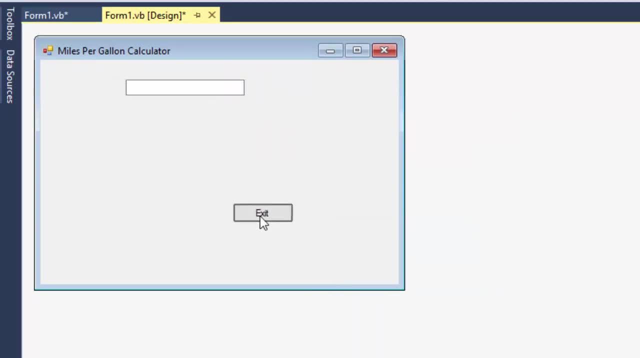 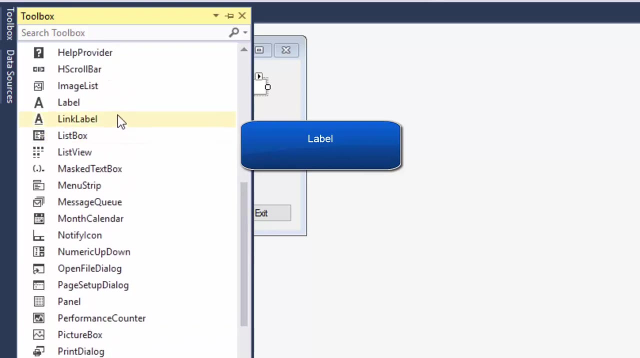 that we want to And that looks pretty good. I can start resizing my form now, because it doesn't need to be massive And I need to let them know what this text box is for. So I'm going to need a label. So I'm going to go over here, scroll up. This is listed in. 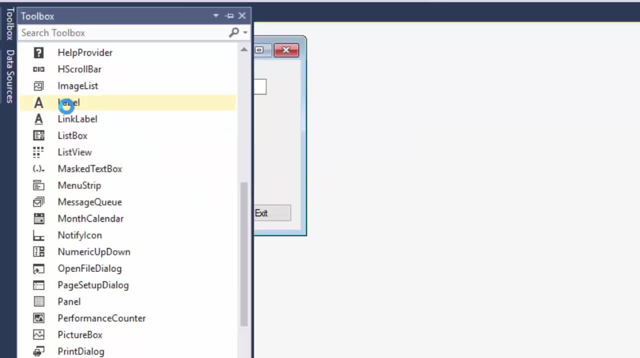 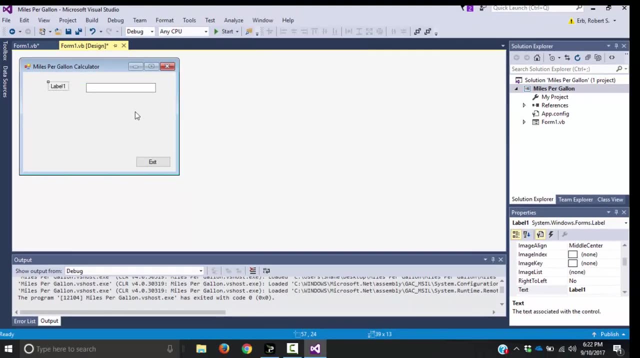 alphabetical order. There's two labels: a label and a link label. Go ahead and click on label. We're not making any Um. I'm going to click on label. We're not making any um. any links here. Drag this label over over, And what I need to do is I need to name these. 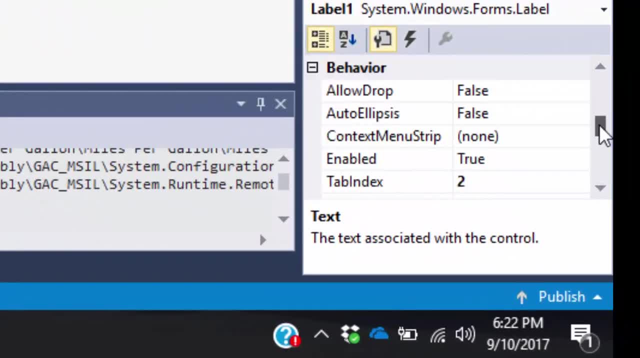 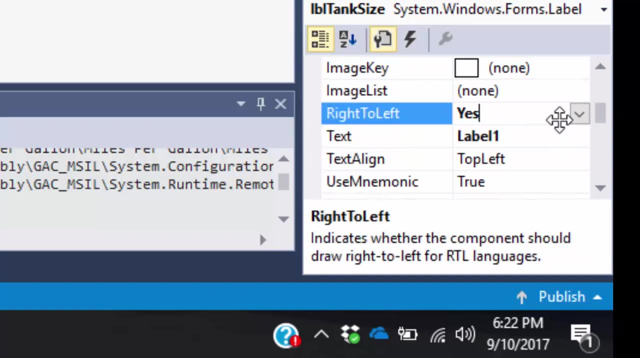 two objects. So this label, we need to change the name of the object And I'm going to say label And we need to know their tank size. So I'm going to call this tank size And what I'm going to do is I'm going to go back up And I'm going to put: uh, change that back. 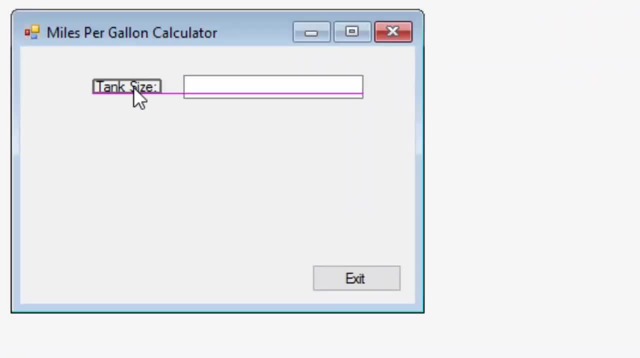 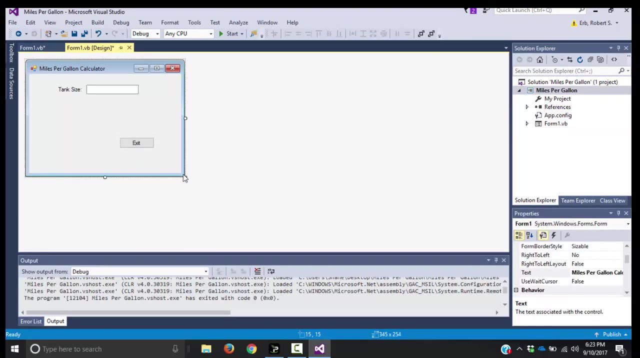 Tank size, And I'm going to put a colon here Now. this lets the user know: Hey, put your tank size right here, Make this a little bit smaller, because it doesn't need to be that big And you can adjust this to however. uh. 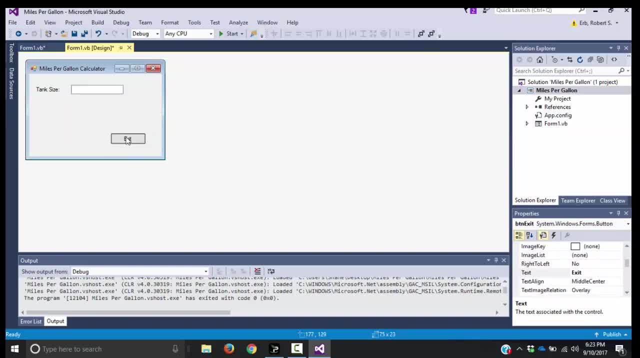 however you would like, You can always do it at the end. I like to do it as I uh, as I go along. just to you know, just to make it look nice, Not too overwhelming, I also need to name this, uh, text box. We're changing the name of the text box from text box to 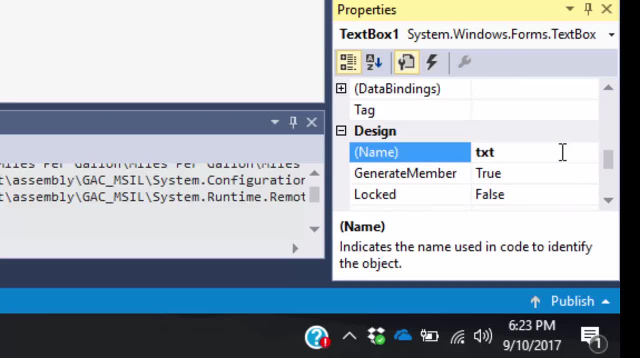 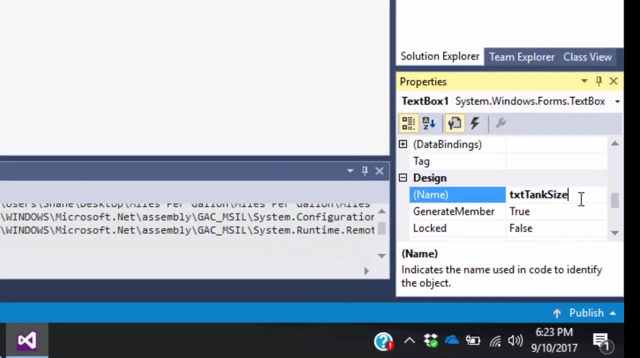 text box. So I'm going to change the name of the text box from text box to text box One, two, T, X, T, which is the prefix, And this is going to be tank size. Now, when you're naming the object, you can not use spaces. If I put a space between tank and size and 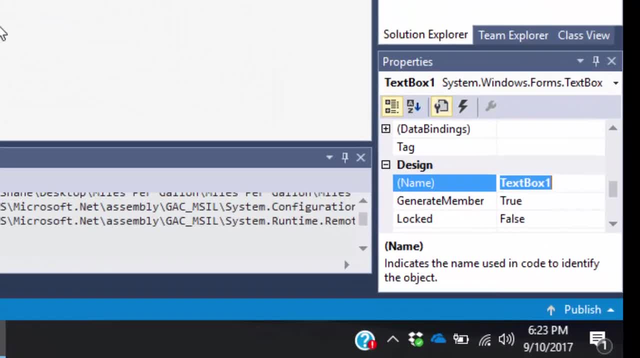 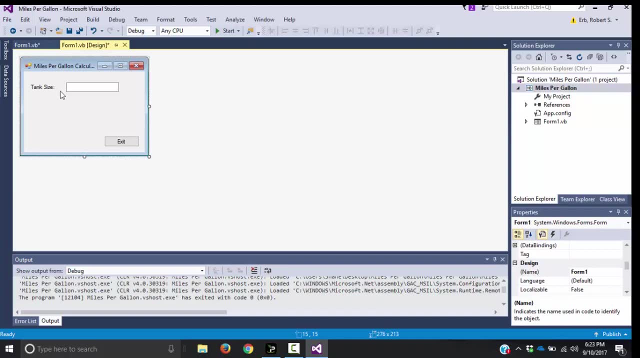 try to use that, it's going to give me an error. So if you're getting that error, it's because you have a space in between. So now I've named it text: tank size. So now that I have these two objects and their names properly, if I want to make it the same size, what I'm 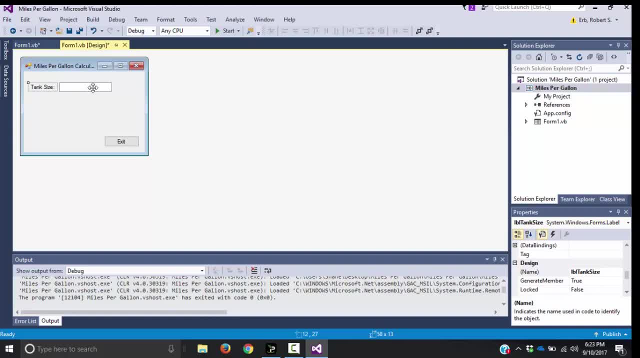 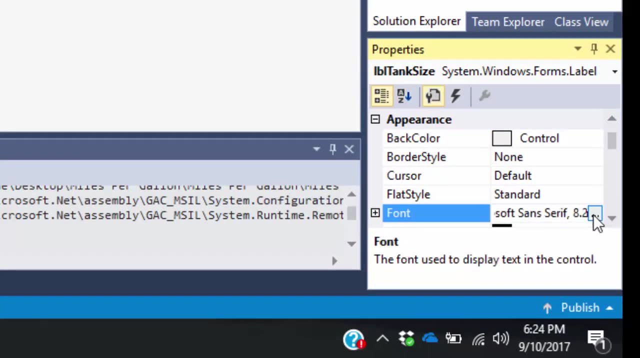 going to do here is: I can um select both of these. I can copy and paste them in, But before I do that, I want to make this label a little bit bigger. So what I'm going to do is I'm going to go to my properties and I'm going to change the font, and you can change. 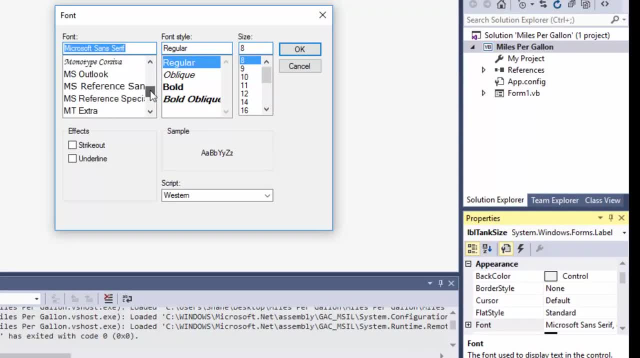 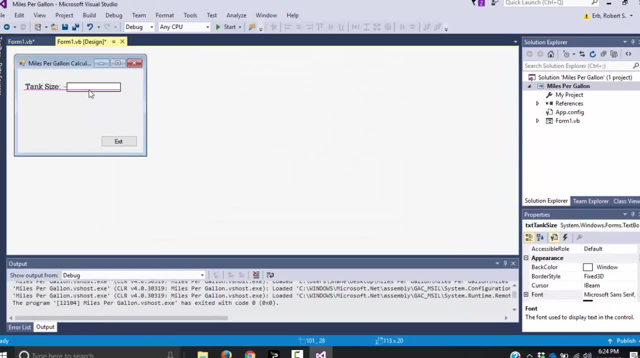 the font to: uh, whatever you want. Um, let's see, here I like to use Rockwell and I'm going to make it about size 12.. Now it's a little bit bigger, You know, a little easier to read. So what I? now that I have what I want, I can hit. 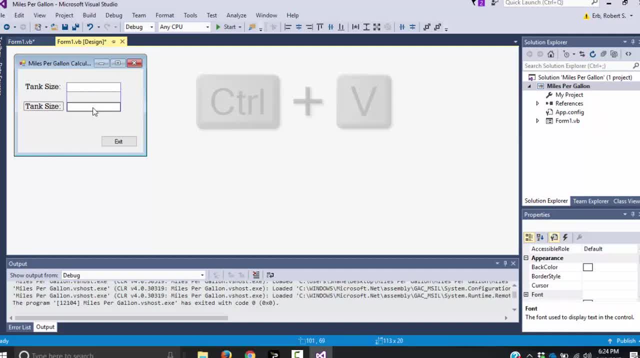 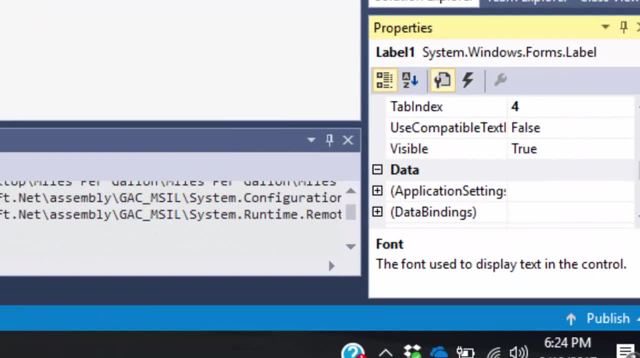 control C, control V, to paste it in. and I need to change the name of this label. So I'm going to scroll down to its name and I just passed it and I need to know how many miles they've gone. So I'm going to call this label miles and then I'm going to scroll up to the text. 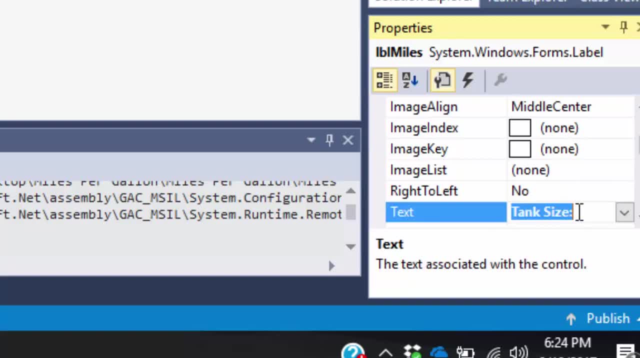 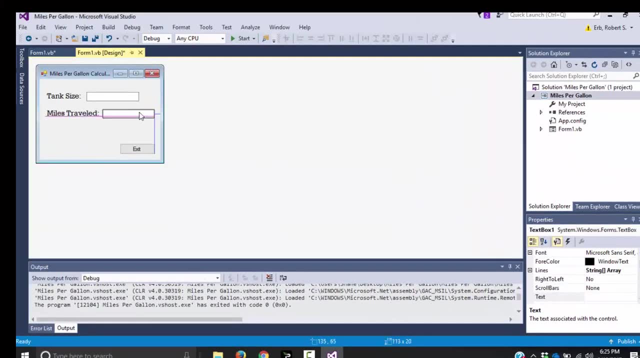 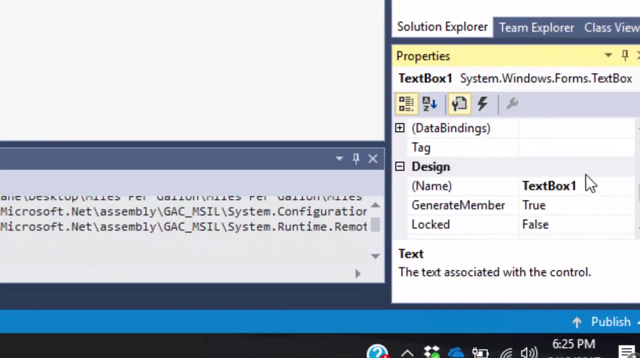 box and I'm going to type in miles traveled, That way we know we want to get how many miles they have traveled. Reorganize this here. That looks pretty good, And the last thing I- or the other thing I need to do, is change the name of this text box, and we're going to change this to TXT. 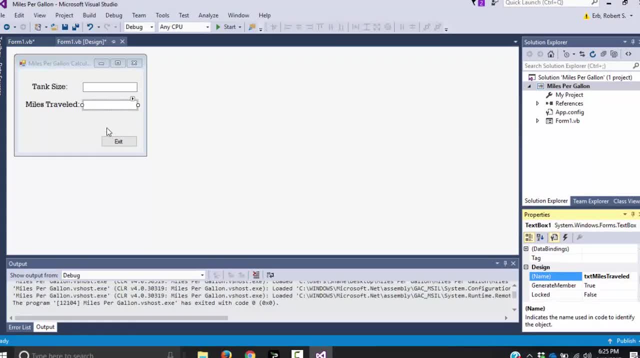 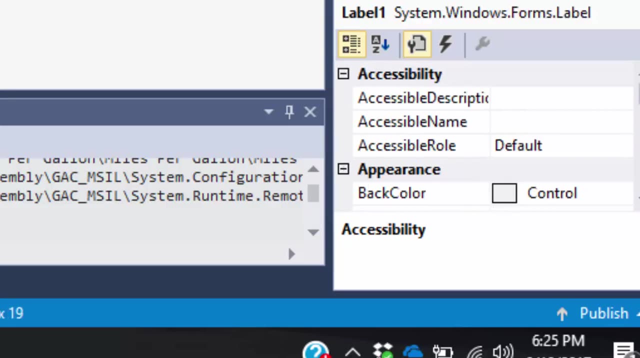 miles traveled. Okay, We need one more uh text box and label, which is going to be the output. So this will be the result. So I'm going to scroll down and change the name. Make sure only one is selected. If you have both selected, the name will not show up. 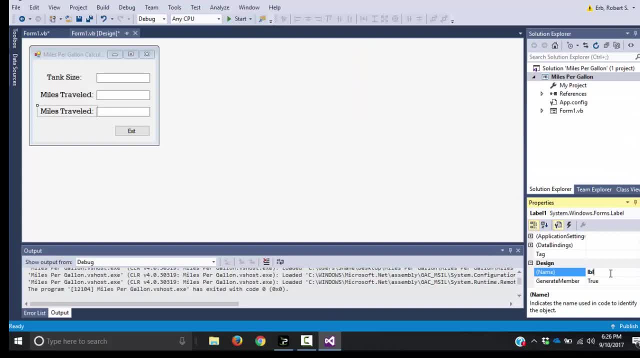 I'm going to change this to label a result, because I'm going to output the result there. I'm going to go here, change the actual text fields to results, put a colon and then I can put that right about there. And then here the text box. I need to change it from text. 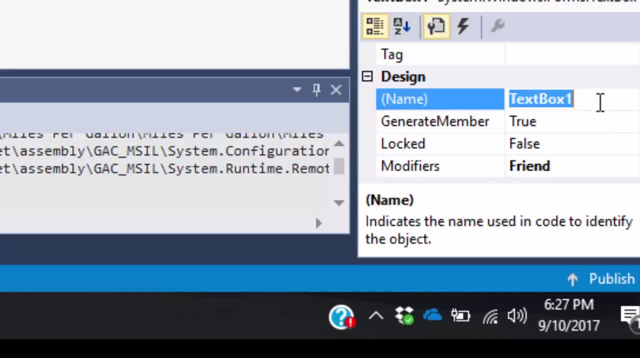 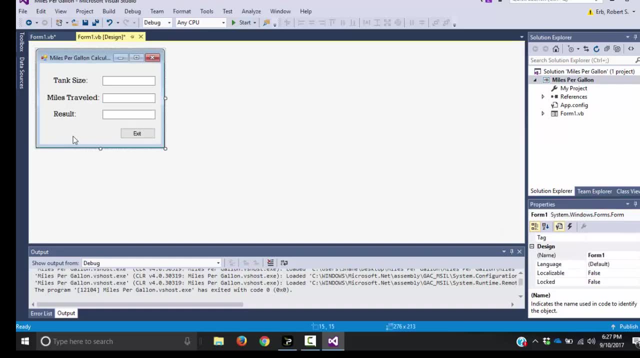 box three to TXT or text box one, because I've already renamed the other two text results. Okay, So I have uh my form here. We can always go back and uh change it later and make it look like however we want. 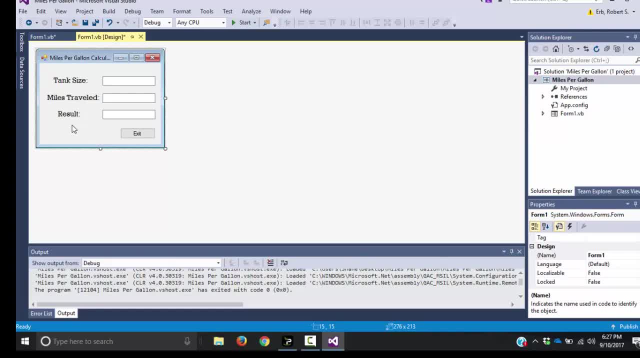 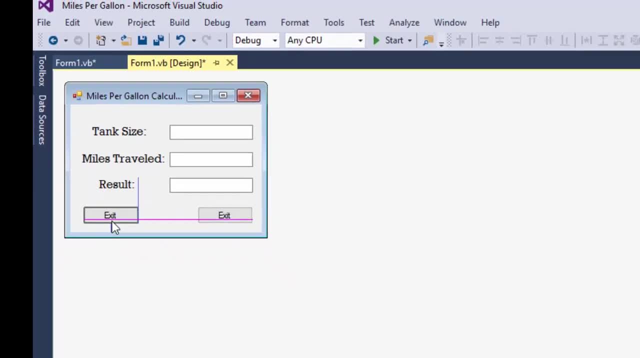 So now what I need to do is actually make it do something, And when I'm looking here, there's one thing I'm missing, which is a calculate button. So I'm going to go ahead and copy this button here and I'm going to change it. It's named to BTN calculate, because 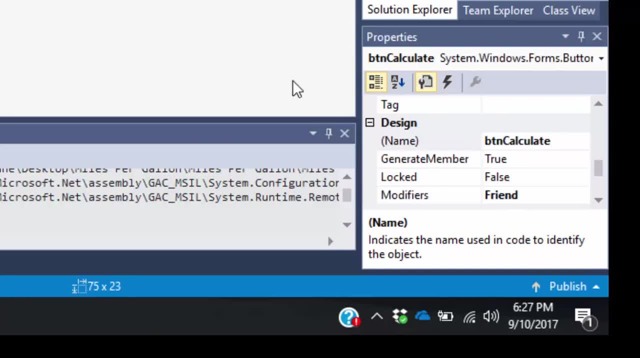 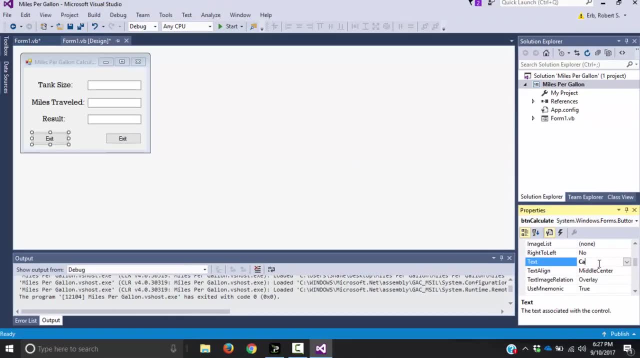 the user needs a way to calculate what they're what they're doing. And then I'm going to go up, change the text field from exit to calculate. Okay, Now I'm looking at this, I'm looking at my form. It looks like we have everything we need. So, uh, we need to do. 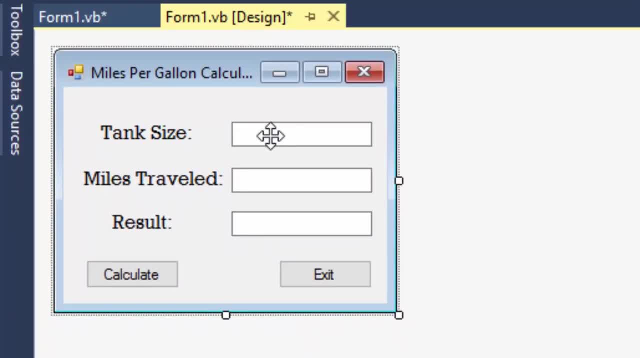 some calculations. Now I don't know what they're going to enter for their tank size, I have no idea what they're going to enter for miles traveled and I don't know what the result is going to be, because it's based on tank size and miles traveled. So this means I need 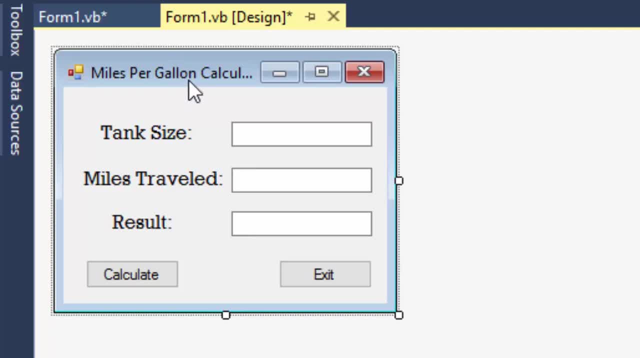 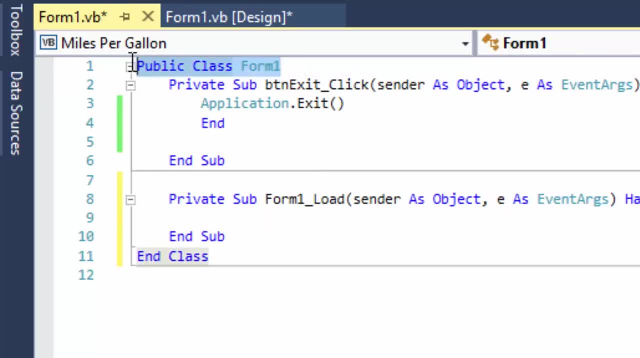 some variables. So what I'm going to do is I'm going to double click my form and this comes up to form load. What I need to do is go to the very top. You'll see we have public class form One. So what I'm going to do is I'm going to hit the enter button. give my self some. 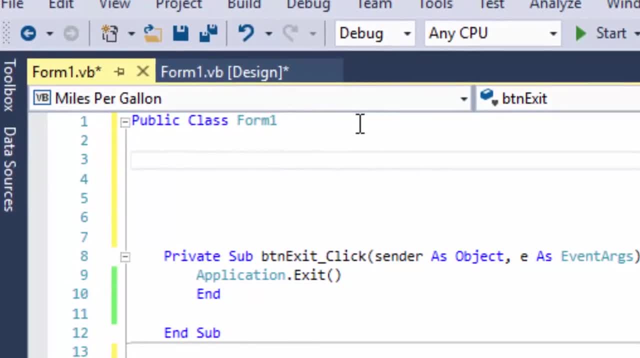 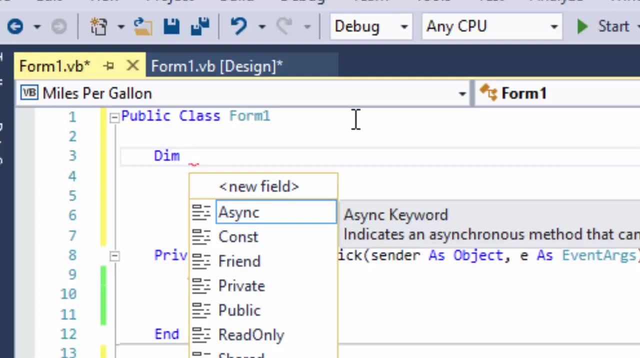 space and some room, And what I'm going to do is I'm going to, I'm going to dimensionalize some variables. Now you might hear some people say dim means dim. I know it doesn't. Dim means dimensionalize. So the first thing we're going to need is a number for the tank size. 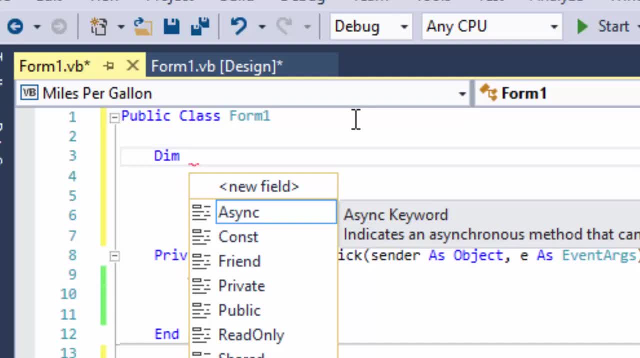 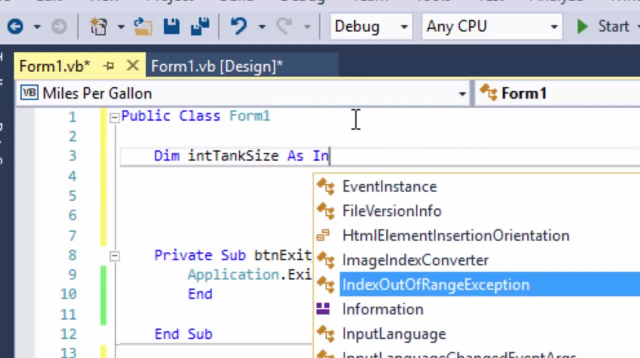 because it's a number. I'm going to dimensionalize that as an integer And there's a prefix we use for integers and that is INT, And then I'm going to do it Tank size as integer Because it's a number I'm going to be working with. I don't have to call it INT, tank size. 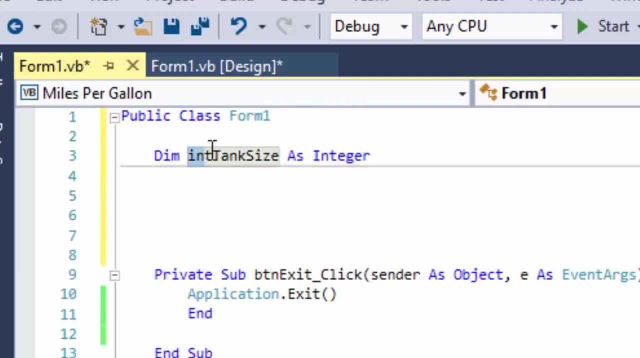 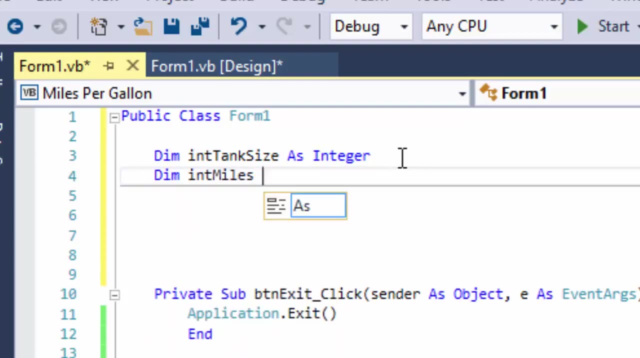 I can call it whatever I want. The INT is standard programming practice to label or to use an abbreviation before each prefix name, So you know what it is. especially as your programs become larger, I'm also going to need another number for the miles traveled. 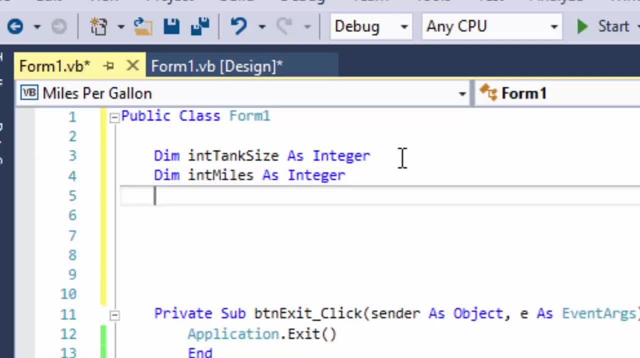 So I'm just going to do dim int miles as integer, And then what I need to do is I need the result, So INT results, as now you might be saying as an integer, but we're not always going to get a whole number. So what we're going to do is, instead of doing it as an integer, 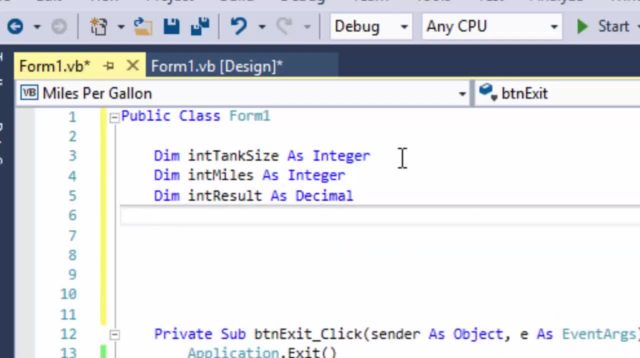 we can still get a number. We're going to do it as a decimal. That way we can get some. if we don't have an exact whole number, it won't round up or down for us. It'll give us a more precise answer, And then the other thing I'm going to need is to make my program. 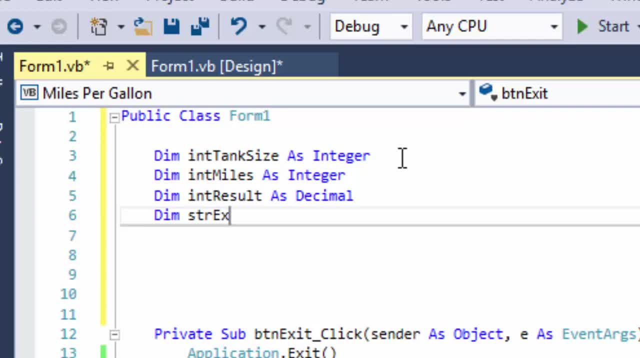 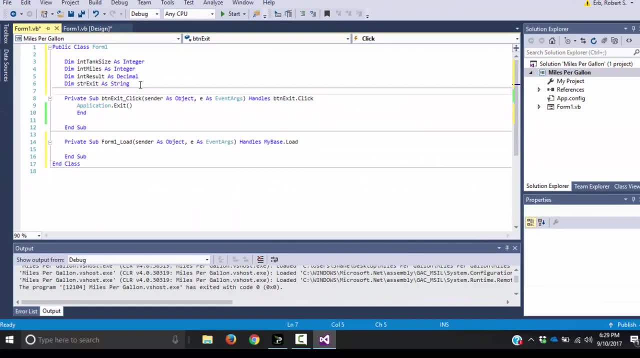 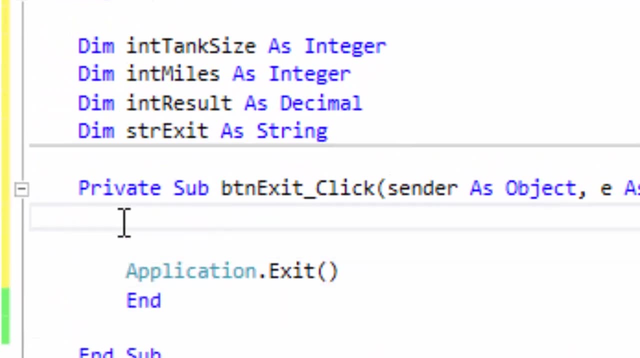 look just a tad more professional- is STR, exit as string, And this is what I'm going to need. I'm going to use cause I don't know if the person really wants to exit or not, So we'll do that right down here. So what I need to do is I need to load, whether or not they want. 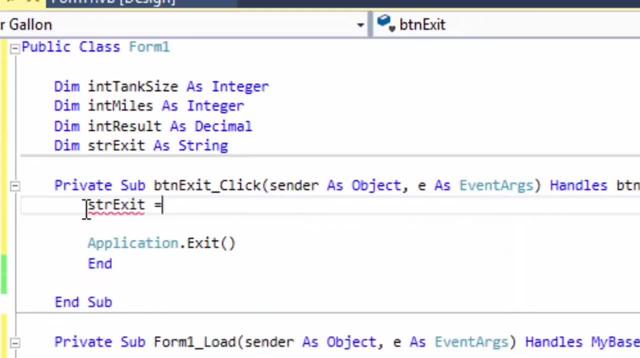 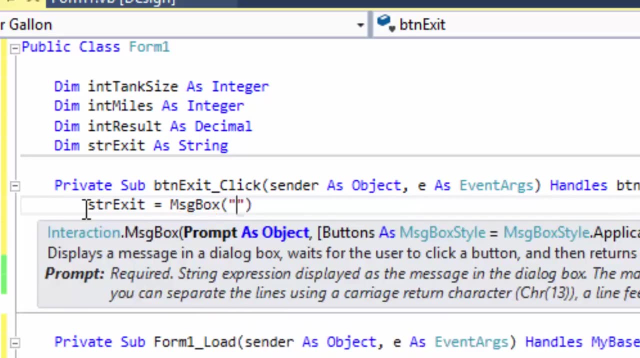 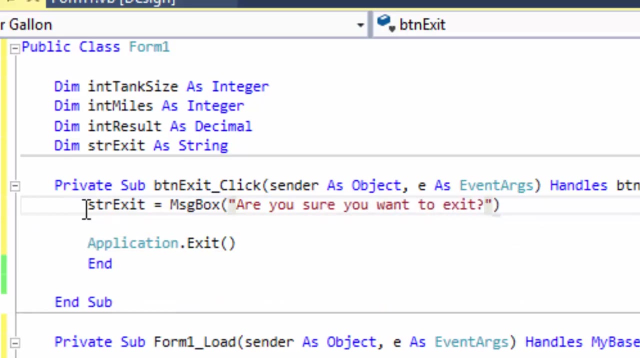 to exit their programs. So I'm going to do STR, exit equals and we're going to create a message box And inside my first set of quotes here I want, I want to ask them the question: are you sure you want to exit? I'm going to go to the end of the quotes. I'm 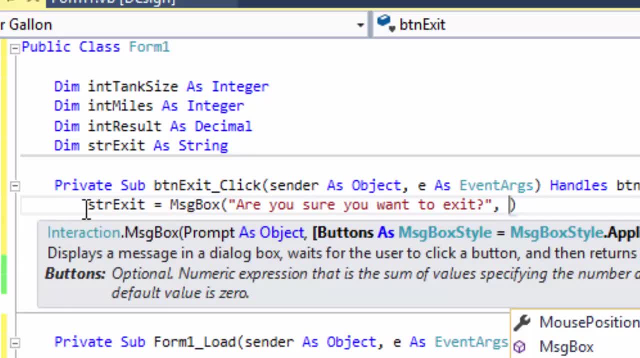 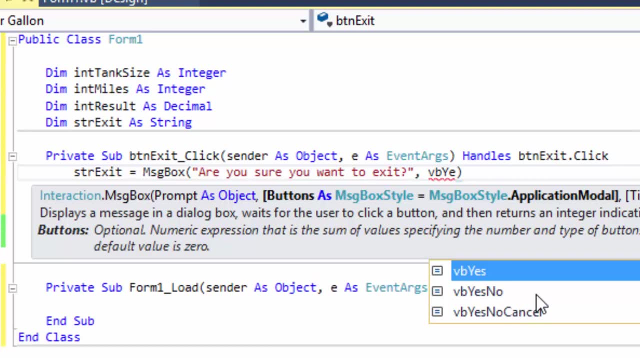 going to put a comment. This will allow me to insert some buttons, So I'm going to do VB, yes or no. We don't need yes, no, cancel. They either do or they don't. There's no reason to have cancel there. 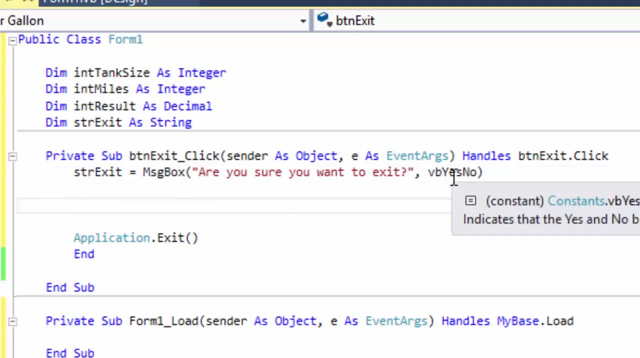 So what happens is, when this message box runs, the user can click yes or the user can click no. depending on which one they, it doesn't matter which one they select. If they hit yes, that's going to be stored in my STR exit variable. If they click no, that's going to. 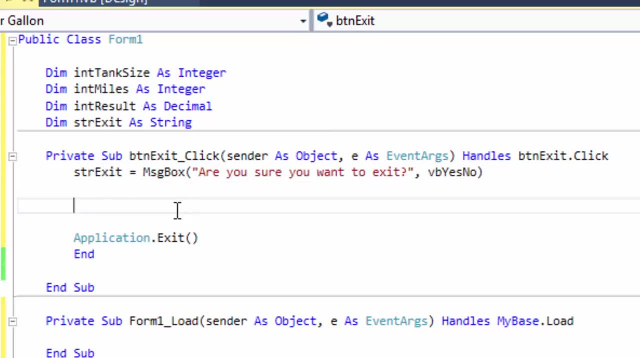 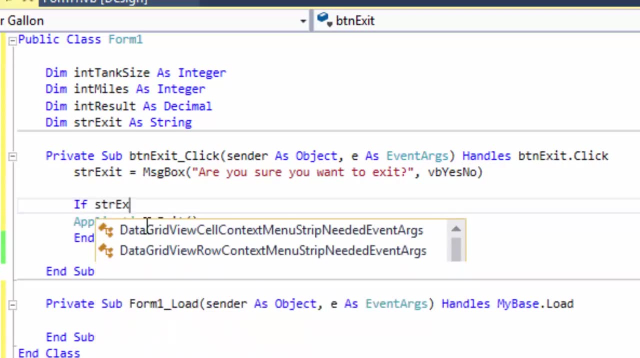 be stored in the STR exit variable. If they click no, that's going to be stored in the STR exit button. If they hit yes, then I want the program to exit. So what I'm going to do is I'm going to create an if statement. If STR exit equals VB, yes then, and I already 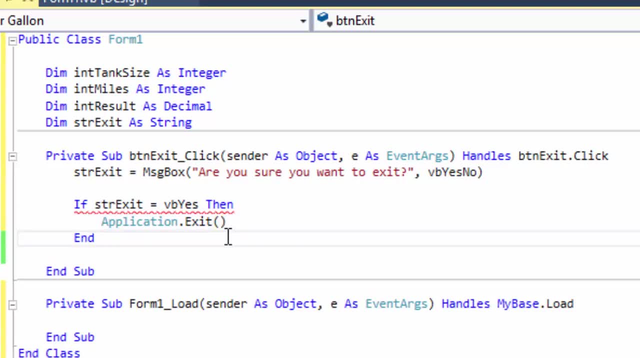 have my code here: applicationexit, end and then end. if So, here's what I have. If they hit yes, which is stored in my STR exit, then we can shut down. If not, the program will keep running, And that's why I have STR exit. So if they hit yes, which is stored, 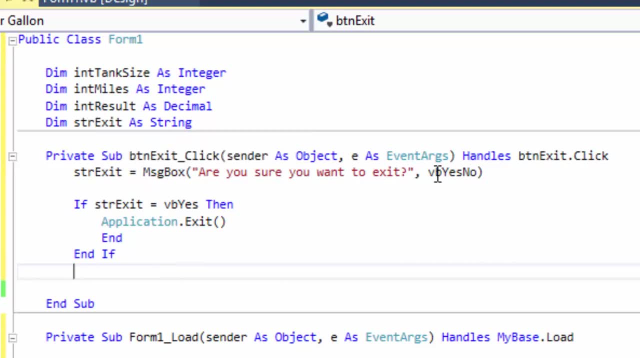 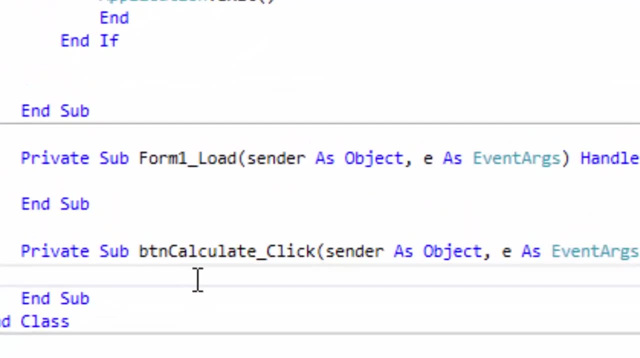 in my STR exit, then we can shut down. If not, the program will keep running And that's why I have STR exit. I got to be able to store. if they put yes or no, All right. so let's do the actual calculating result. I'm going to double click on calculate. I'm on. 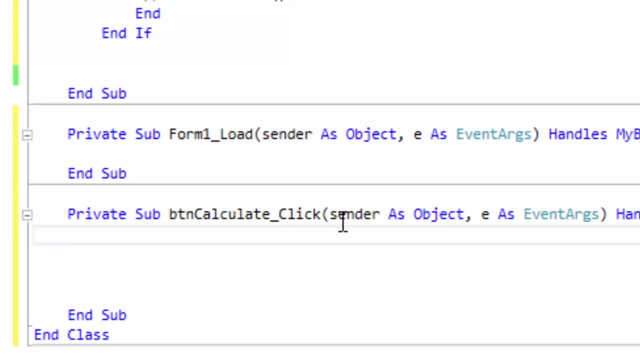 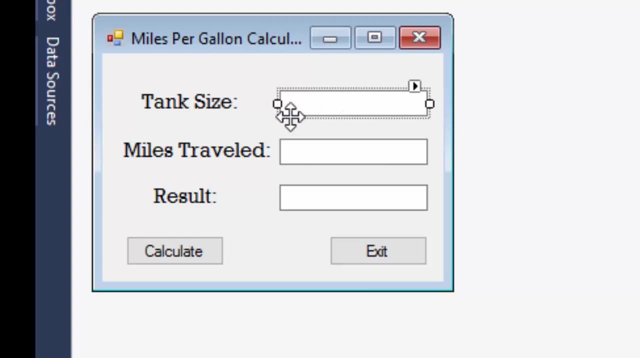 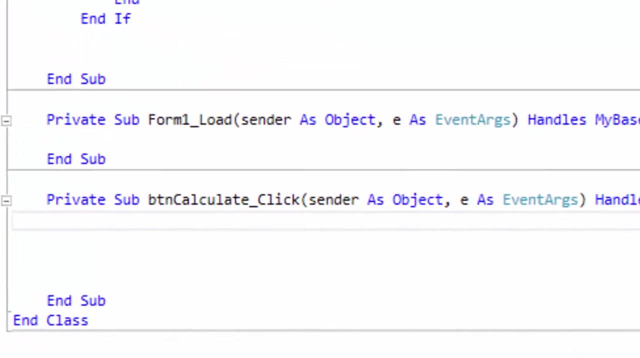 my button calculate click. So here's what we're going to do: We need to take whatever is in this text box and store it into the tank size variable. We need to take whatever is in this box text box and store it into the mils variable. So what I'm doing is I'm taking my variables that I just created And I'm going to take this particular variable. I'm going to review Tampa Bay. Okay, I just take this copy And I'm going to reduce my new information that I just created And I'm going to remove some of the comprised information. 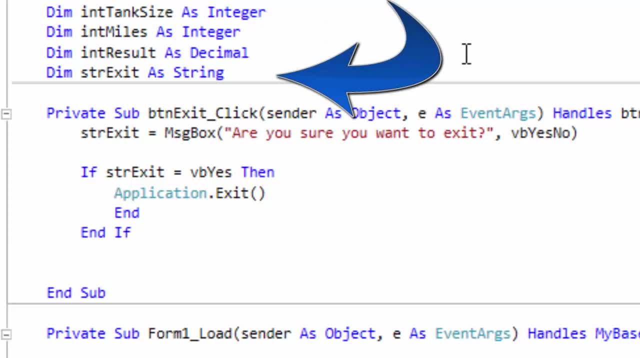 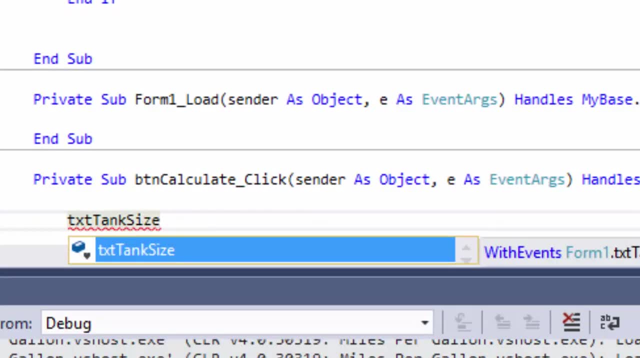 and I'm going to go right into the others together. So if they want a вот and all, I just- And I'm fixing to store something in the both of them When they click calculate. I'm going to take text tank size And this is why we rename text boxes rather than leaving it text box one. we know what we're working with here. So when you do text tank size, dot text, you need to have that there because you have to select the property, And what we're going to do is we need to store that inside of a variable. Because we're storing it inside the variable, we need to put the variable on this size. 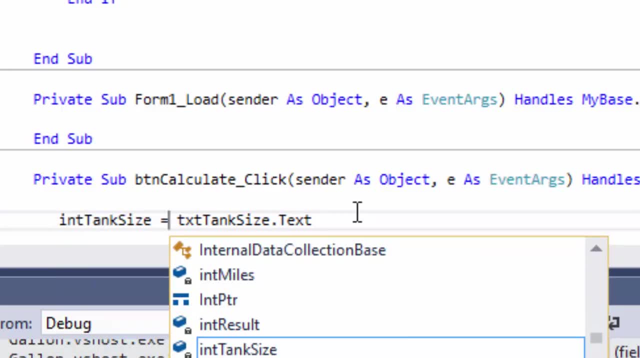 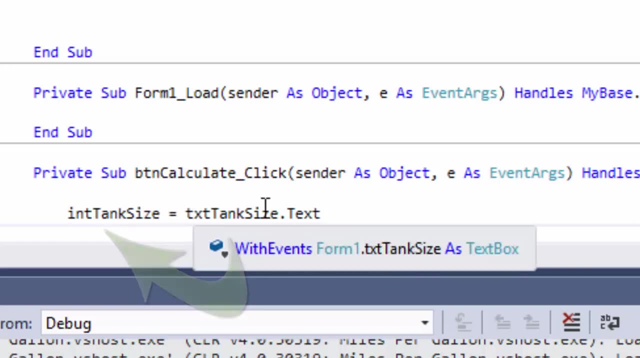 On this side. Alright, so when I look at this, here's how it's read. Whatever is here is going to go into what is on the left hand side. So I'm taking what is inside the text box for tank size, I'm storing that in to the variable And I need to do that for the miles as well. So int miles equals txt miles traveled And I can't leave just text miles traveled. There's lots of properties. I need to let the program 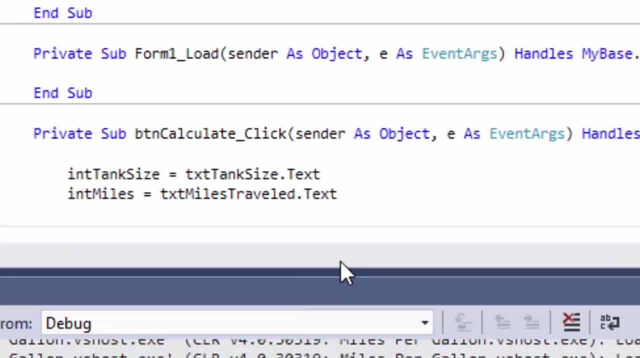 know which property and I want to use the text. Now, once I have that, I need to do something with it. So I have these two numbers because I took what was in tank size text box. I stored that. So this variable is holding a number. I took what's stored in this text box, put it into int miles variable. it's holding a number, So I need to do something. So I'm going to take my int result And what I'm going to do is I'm going to take my miles traveled. 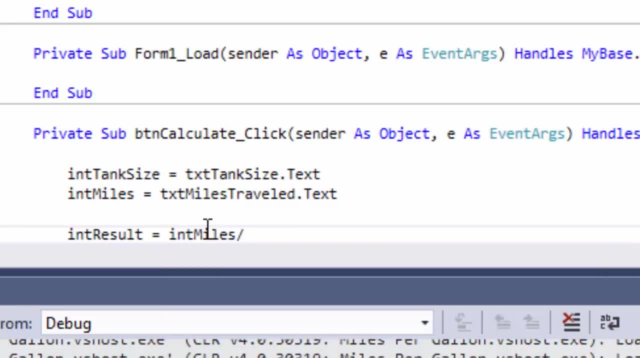 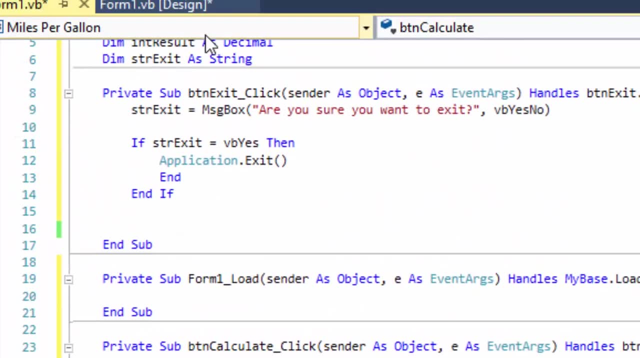 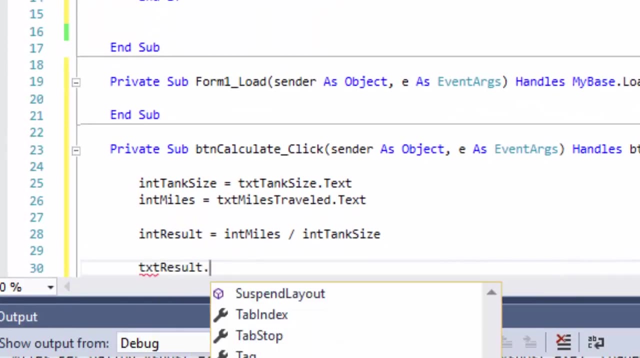 and I'm going to divide that by the int tank size. So that's going to give me a result. However, I need to put this result inside this text box. So what I'm going to do this time is I'm going to do: text result dot. txt equals int result, And here's what happens: I have to use this calculation First. once I use this calculation and get the results,